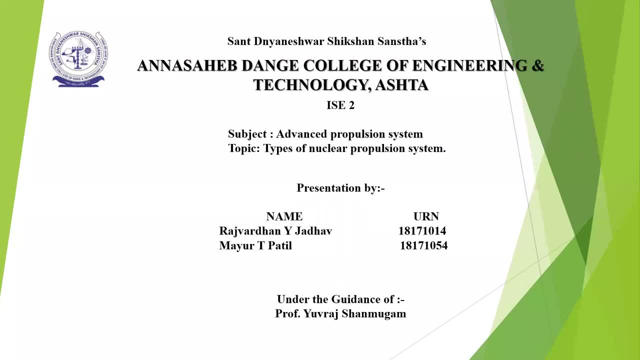 Hello friends, my name is Rajavurthi Nishwantzathu and I am from Anna Sahib Dangay College of Engineering and Technology, Ashta, and subject is advanced propulsion system and for our today's presentation, our topic is types of nuclear propulsion system and my group member is Mayur Patil and we prepare this presentation under the guidance of Professor Urashan Mughansar. 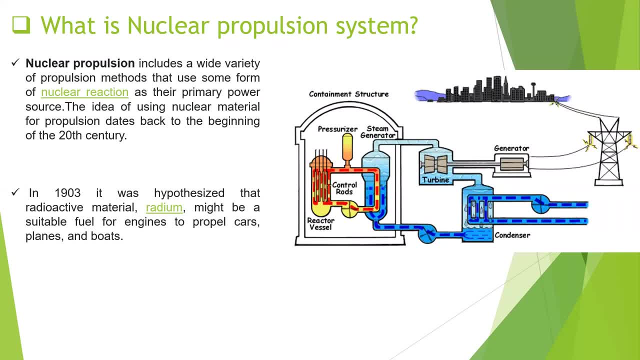 So first, here we see the what is the nuclear propulsion system? Nuclear propulsion includes a wide variety of propulsion methods that use some form of nuclear reaction as their primary power source. The idea of using nuclear material for propulsion dates back to the beginning of the 20th century. In 1903, it was hypothesized that radioactive material, radium, might be a suitable fuel for engineering to propel cars, planes and boats. In this diagram we see the 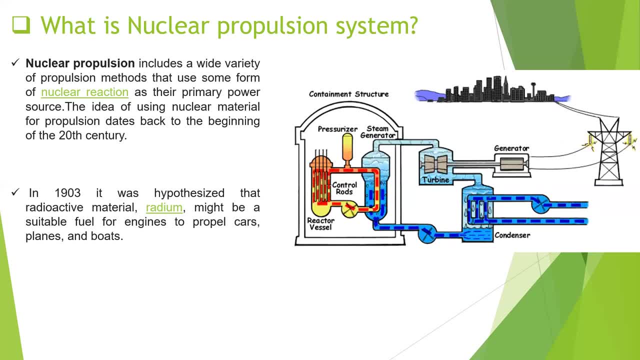 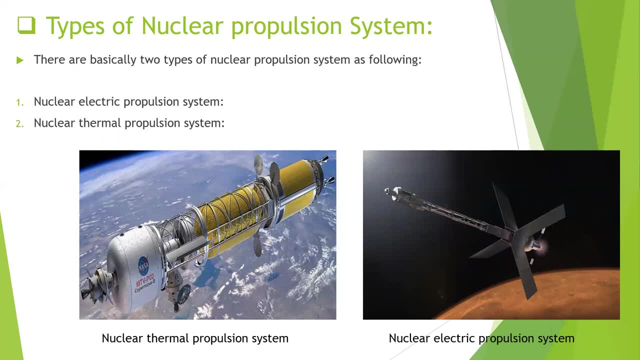 where this is the basic diagram of the nuclear propulsion system. Now here we can see the types of nuclear propulsion system. There are basically two types of nuclear propulsion system, as following: First is nuclear electric propulsion system and second is nuclear thermal propulsion system. Here we see the conceptual diagram of both propulsion systems. 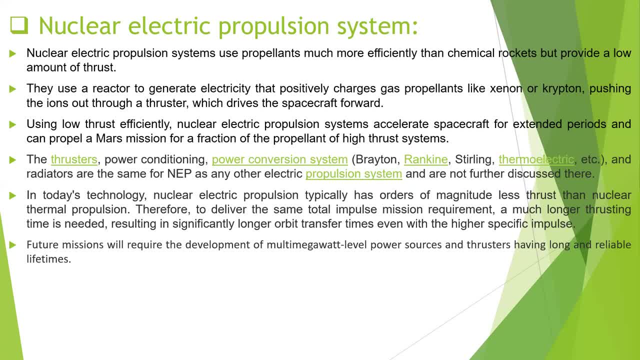 Now here. first we see the nuclear electric propulsion system. Nuclear electric propulsion system is a type of nuclear propulsion system. Nuclear electric propulsion system use propellants much more efficiently than chemical rocket, but provide a low amount of thrust. They use a reactor to generate electricity that positively charges gas propellants like Xenon and Kryptor, pushing the ions out through a thruster which drives the spacecraft forward. 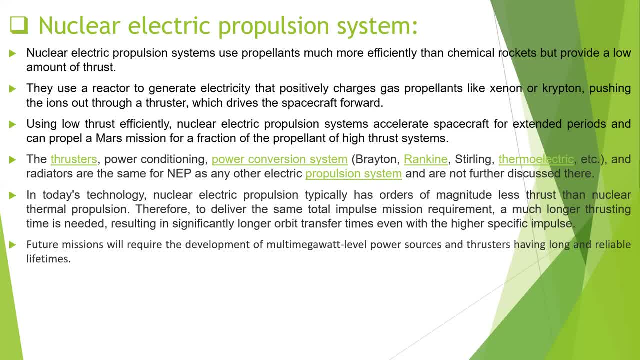